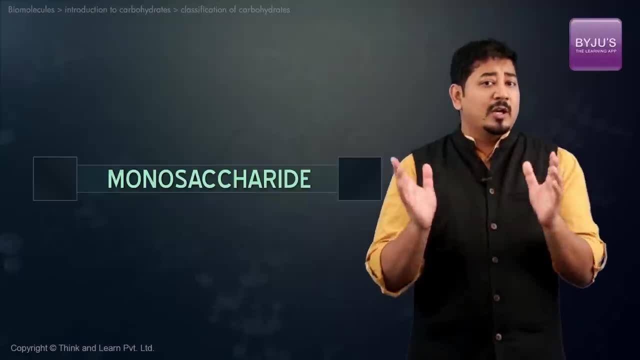 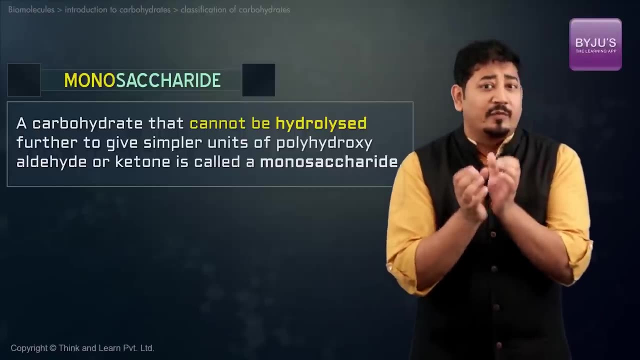 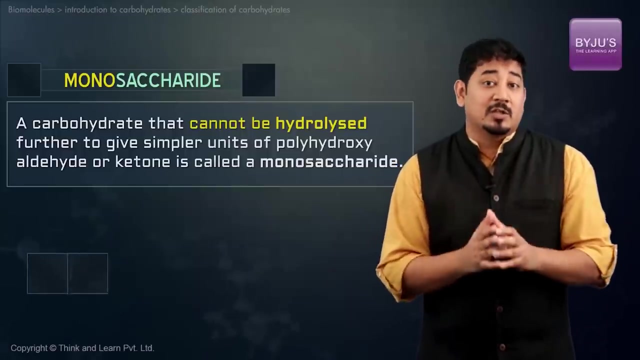 monosaccharides. Look at the clue in their name. The keyword here is mono, or one A carbohydrate that cannot be hydrolyzed further. to give simpler, units of polyhydroxy aldehyde or ketone is called a monosaccharide, As the name suggests, they are made up of just one saccharide unit. 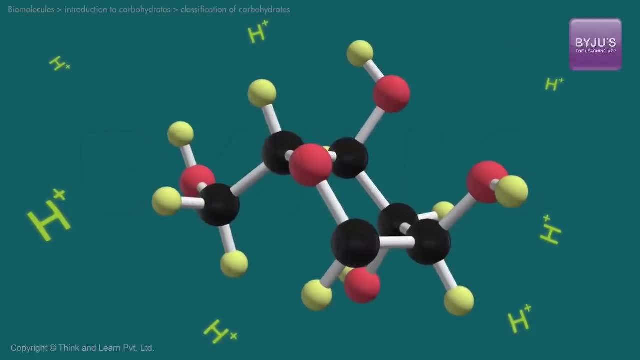 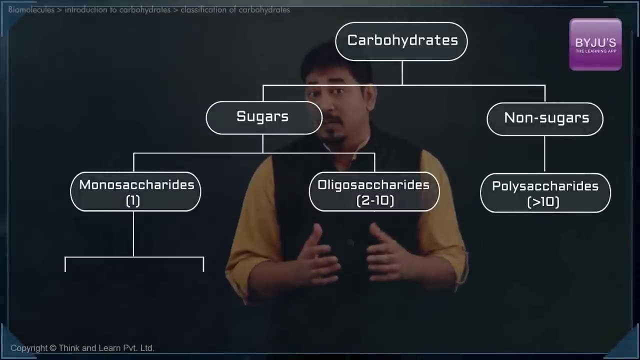 Simply put, we cannot use water to break these down into smaller units, because these are the smallest units that we can have Now. they can be further classified depending on whether there is an aldehyde group here, which is, in this case it's known as an aldose, or if it has a ketone. functional group, in which case it is known as ketose. About 20 monosaccharides are known to occur in nature. We will look at the names and structures of these very soon. Let's now move on to oligosaccharides, though Carbohydrates that yield 2 to 10 monosaccharide units on hydrolysis. 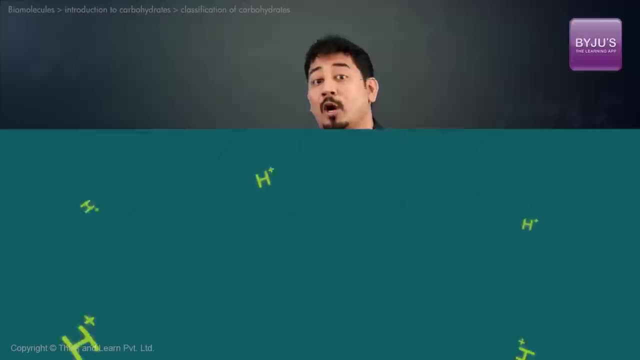 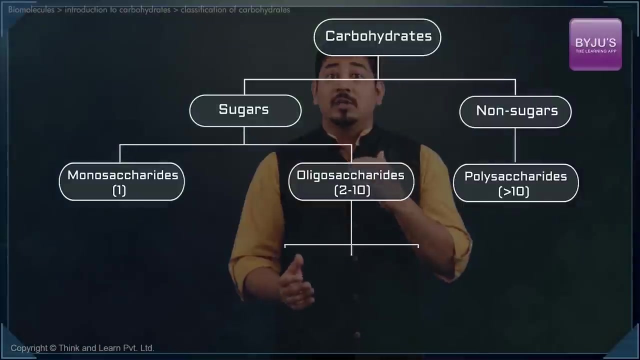 are called oligosaccharides. This means that water is able to break these compounds down to smaller units, which are in turn monosaccharides. Now these can further be classified based on the number of monosaccharide units it produces on hydrolysis. So you can have 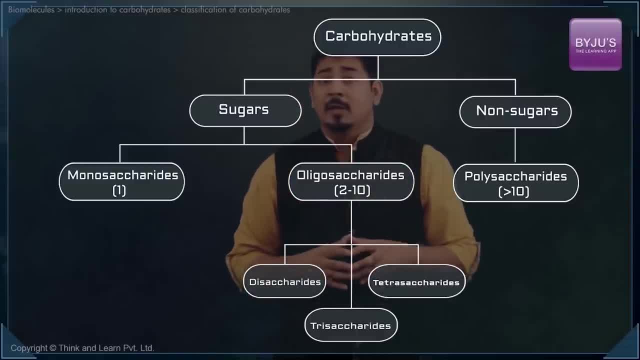 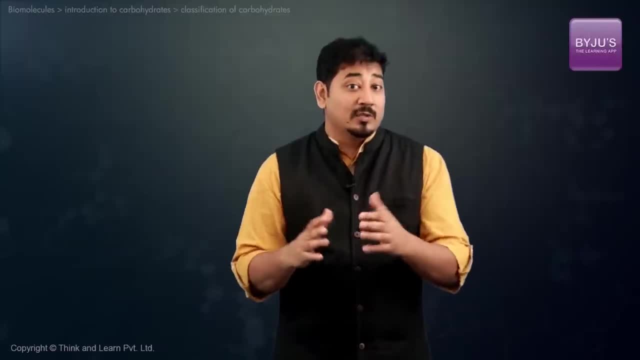 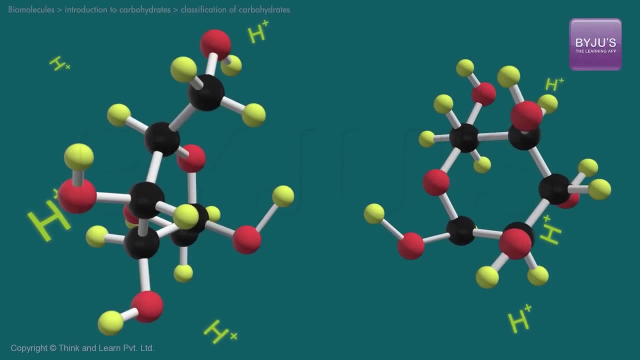 disaccharides, trisaccharides. you get the idea right. The most common ones among these are disaccharides. Now, it is important to mention here that the monosaccharide units we get after hydrolysis may not always be the same one. For example, sucrose, a disaccharide gives glucose. 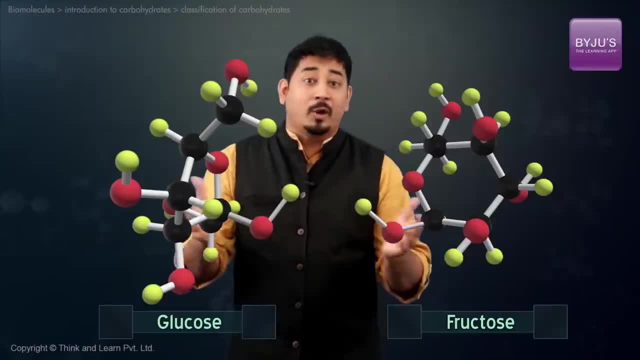 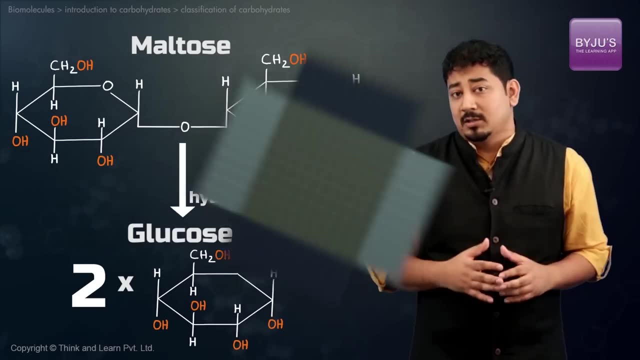 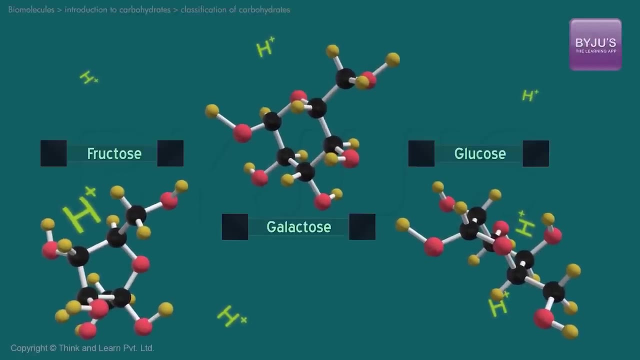 and fructose, which are two different monosaccharides, upon hydrolysis. But maltose, which is also a disaccharide, will give you two units of glucose on hydrolysis. A common example of a trisaccharide is raffinose, which gives galactose, glucose and fructose on hydrolysis. Now there are 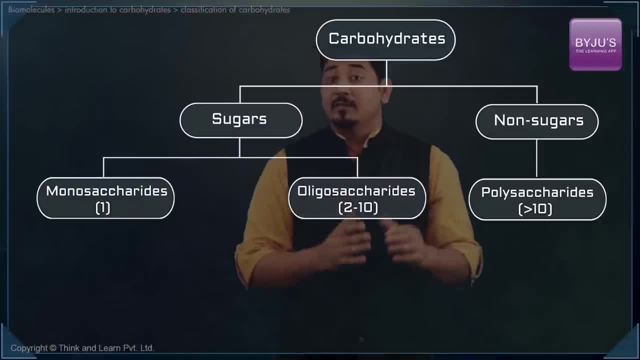 many such examples of oligosaccharides. Finally, we have carbohydrates, which yield a large number of monosaccharide units on hydrolysis. These guys are called polysaccharides. Some common examples here include starch, cellulose, glycogen gums, etc. 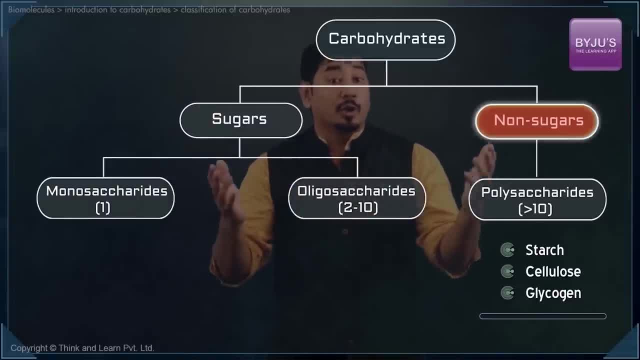 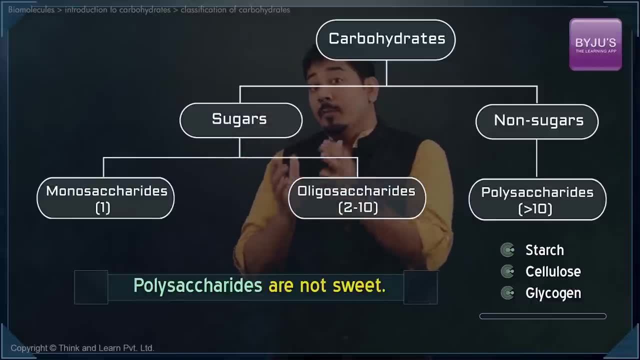 Now, if you look at the table, you see that polysaccharides are put under non-sugars, whereas monosaccharides and oligosaccharides are put under sugars, And this is precisely because there is no polysaccharide, which is sweet in taste. So all polysaccharides as such. 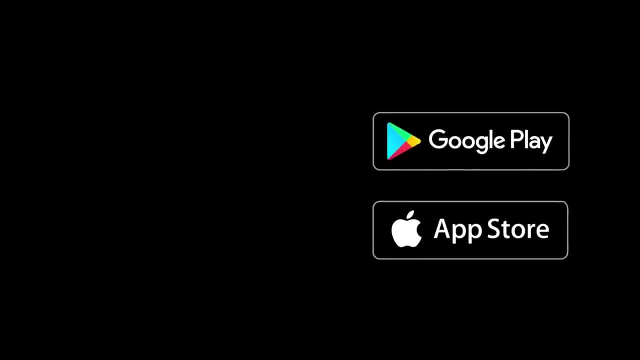 are non-sugars To keep learning with such engaging videos. download Byju's the learning app today.